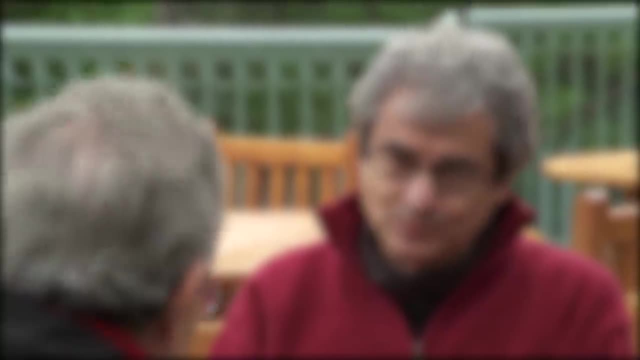 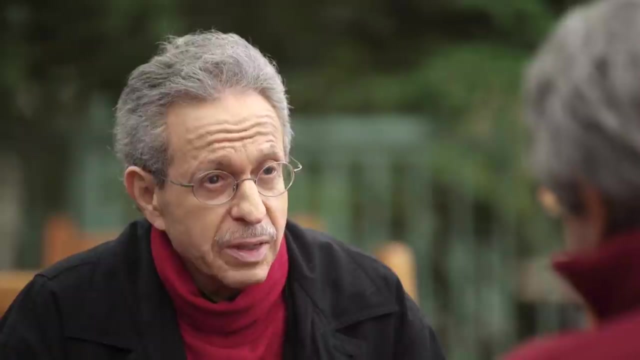 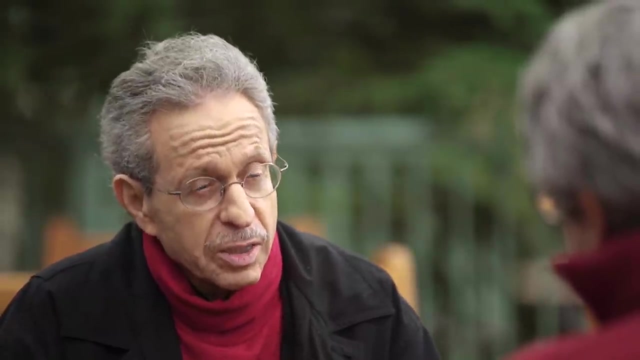 Carlo, one of the pinnacles of human achievement is being able to unify the understanding of the most small in quantum theory with the most large, which is the origins and structure of the universe. As someone who works in quantum cosmology, what are your emotions and what? 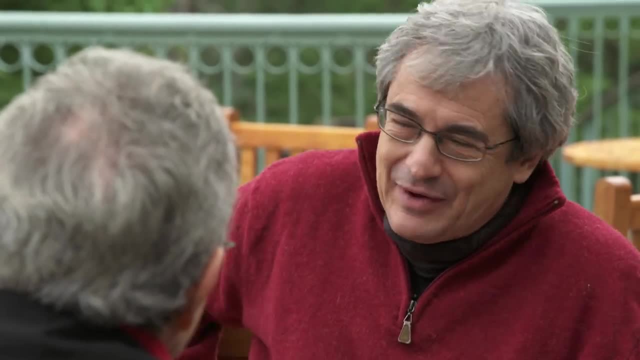 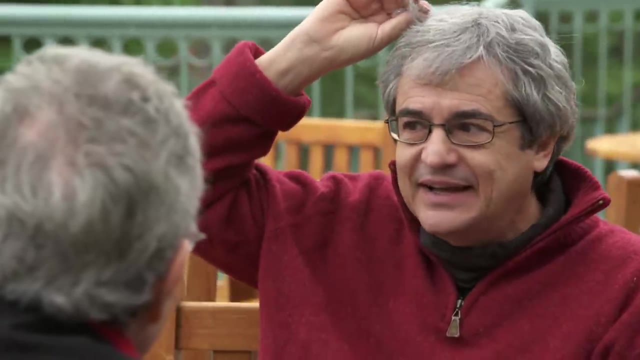 are the kinds of things that you do. My emotions is that it's infinitely charming and a fascinating question. I mean, I'm infinitely attracted to it. I think it's important to separate problems, not to confuse problems. Quantum cosmology is a name which is a bit too. 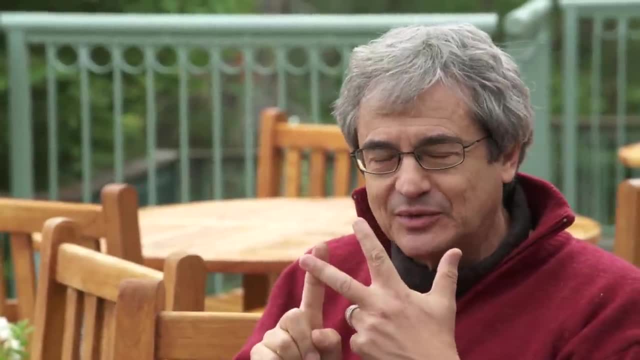 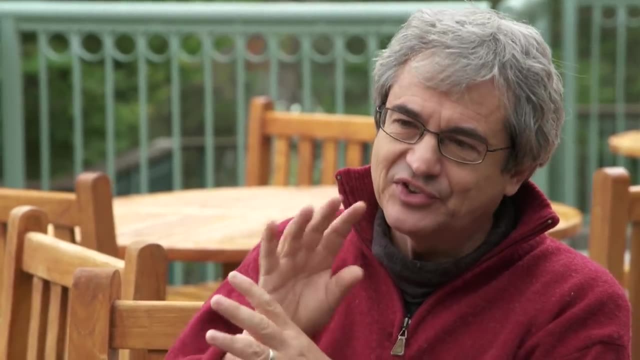 vast. I think one separates three different problems, and one is quantum gravity. Quantum gravity by itself has nothing to do with cosmology. So quantum gravity is a problem. what are the quantum features of space and time, or the gravitational field? We know the. 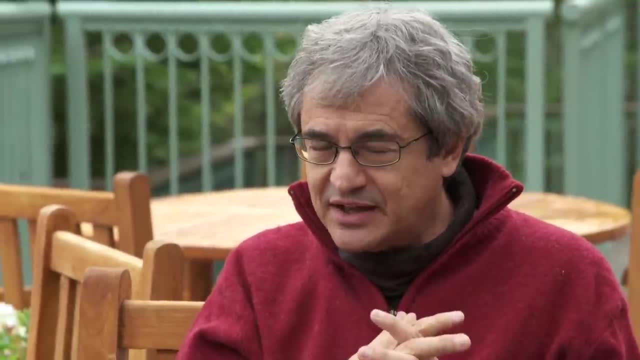 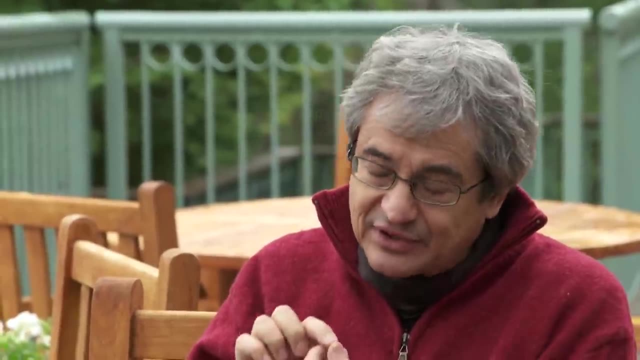 gravitational field is spacetime, So what is the quantum property of that? So if I ask what happened to the center of a black hole, it's going to black hole explode or whatever. If it happened that space is granular, as I believe in loop quantum gravity, that would be. 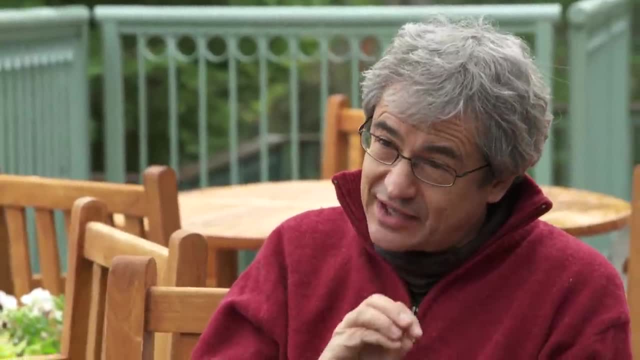 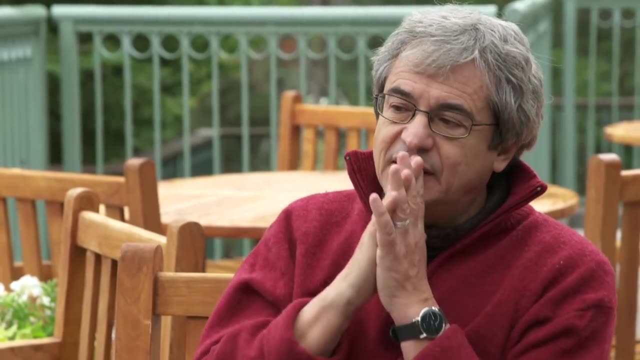 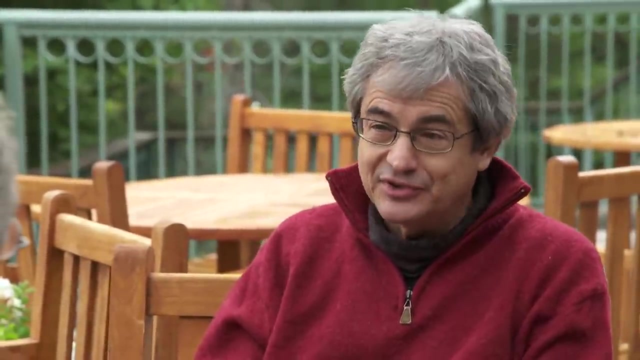 fine. These are quantum aspects of space and time, of gravitational field, nothing to do with the cosmos. So that's one, it's quantum gravity. Number two is we see the universe expanding. We have this marvelous thing which is scientific cosmology, started by Einstein. with all these, 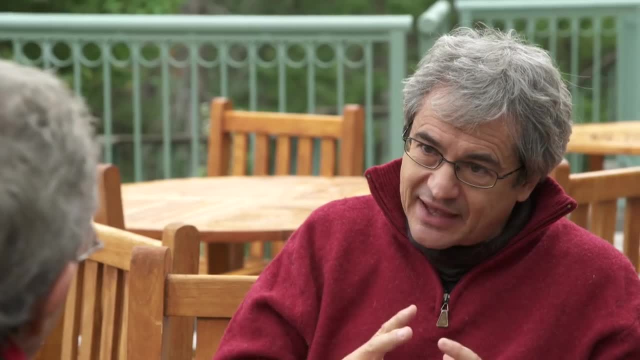 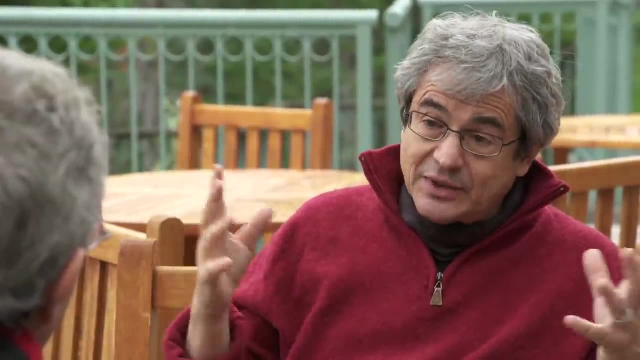 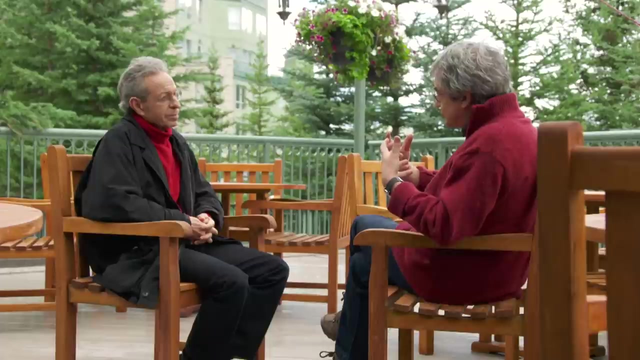 observations. We see the universe accelerating. we realize it was a big bang, Fantastic. There's a dynamic of the big thing. This dynamic of the big thing needs quantum mechanics. Why? Because in the deep past there was probably quantum. so we need quantum gravity, So we need quantum gravity. 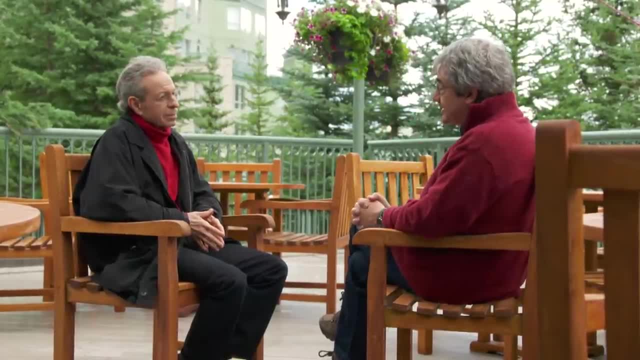 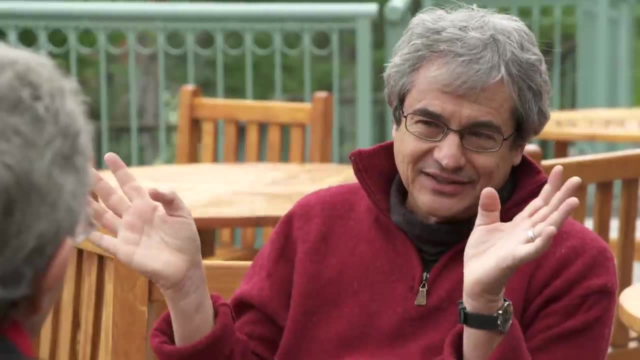 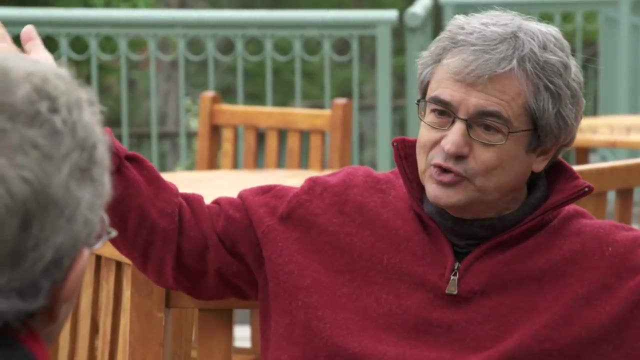 to understand the quantum aspect of large structure, And that's quantum cosmology one. Quantum cosmology two, which is a totally different thing, is: how do I do the quantum theory of everything? But everything doesn't mean the universe at large, because what the cosmologist studies is the universe at large, which doesn't mean 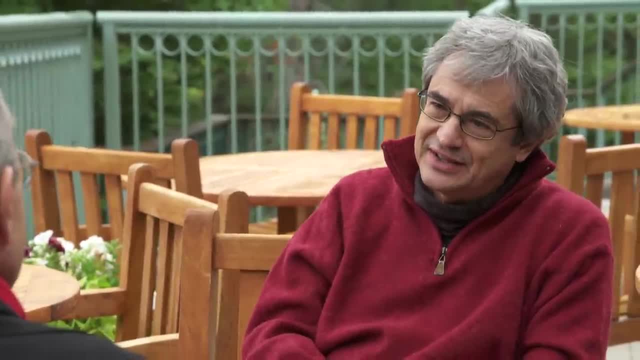 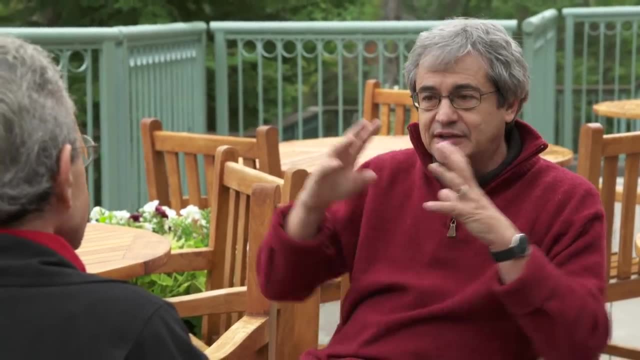 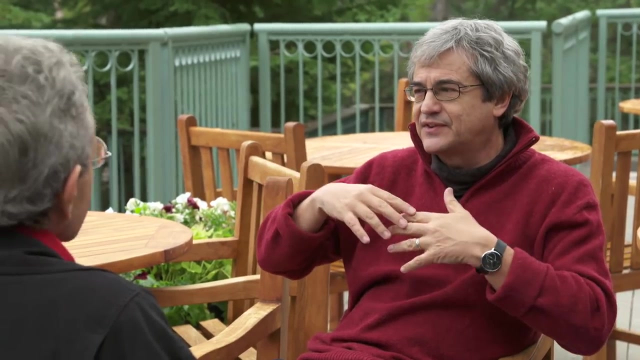 for instance you and I. You and I are not in the equation of the cosmologist. My little finger is not in the equation of the cosmologist. So cosmology is the study of large degrees of freedom of the universe. Quantum cosmology sometimes is used in the sense of 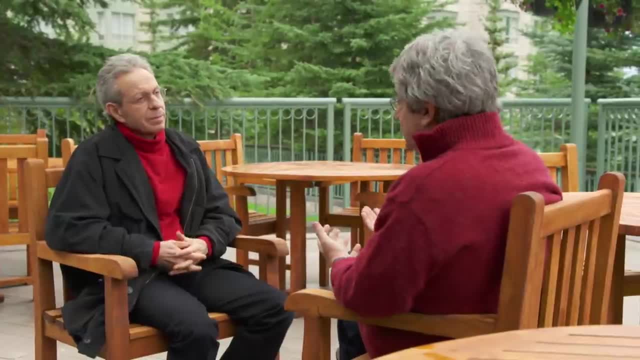 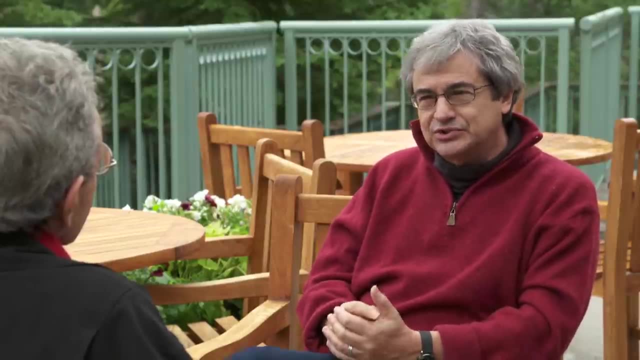 the quantum theory of everything, which would be a good problem even if the universe was not expanding, even if there was no big bang. And I think the quantum theory of everything is a premature problem. We don't have clear ideas about that. We're confused about quantum. 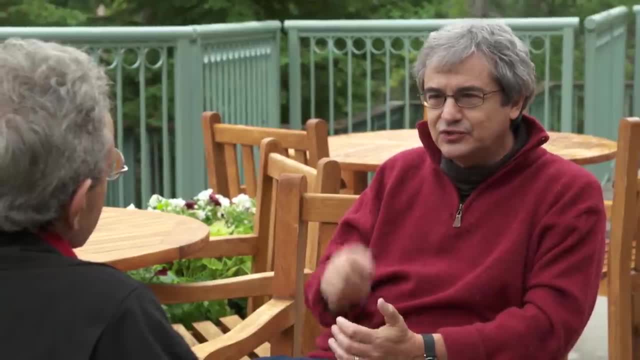 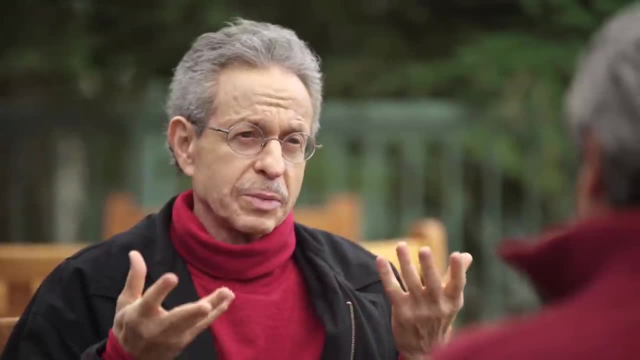 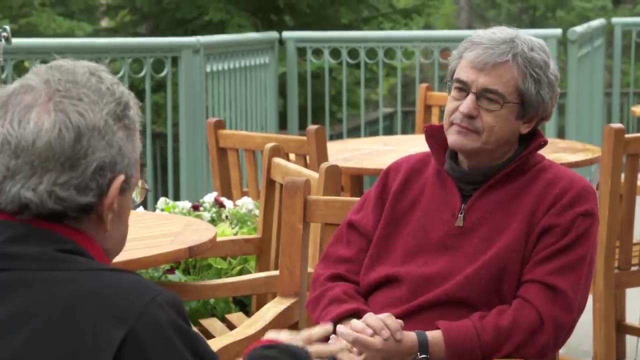 mechanics. We should not confuse the three problems. These are three very different problems. What is the unity in terms of the thinking that's brought to the three problems? It's obviously an idea of the world in quantum terms. There's some basic thing underlying all three. 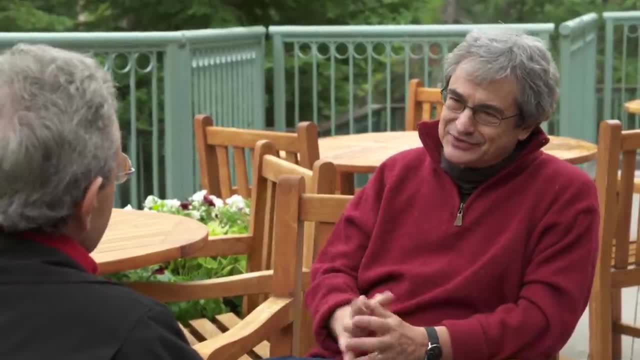 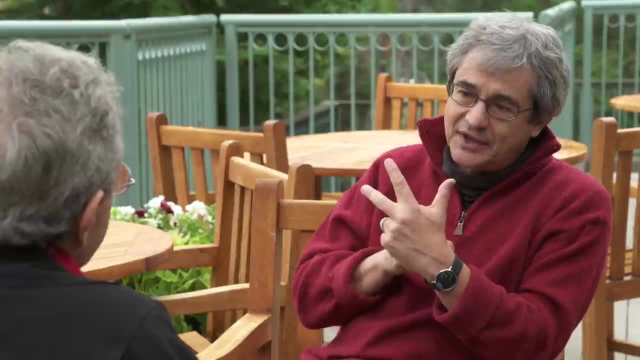 Yeah, We do believe that quantum mechanics is the basic theory of how things move, how things happen, how things change. So three things have happened: One is the discovery of quantum mechanics, One is the discovery of generativity And one is the beginning of. 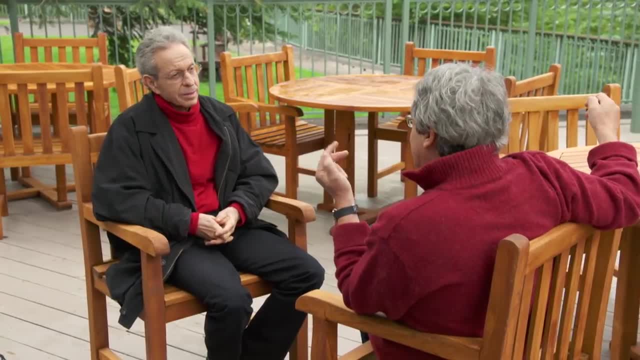 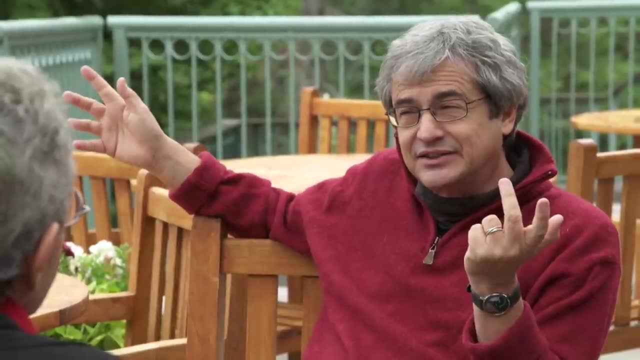 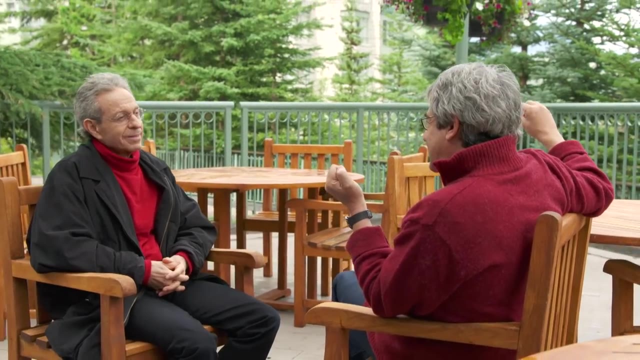 the scientific study of the large scales. Nobody thought really that it was possible before 1917, when Einstein published this incredible article. It's a fantastic article because it's one of the best Einstein articles and it's full of mistakes. He says: obviously the universe is not expanding. 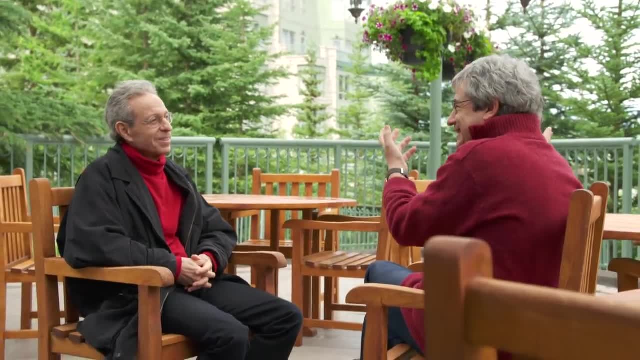 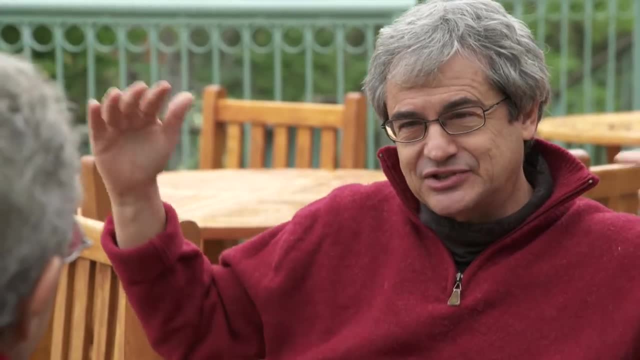 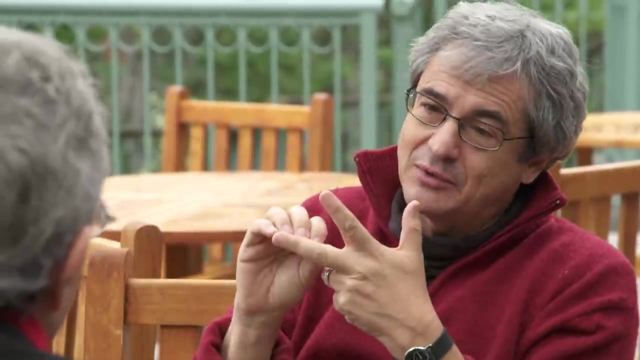 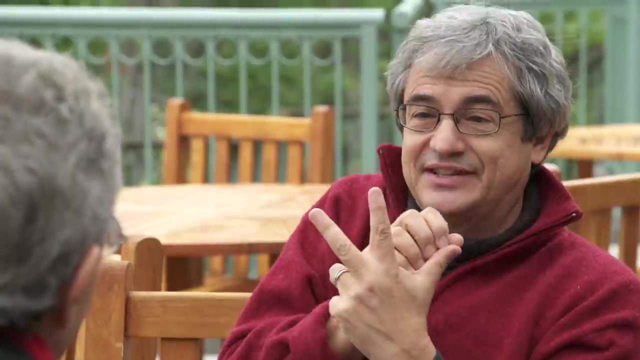 and therefore this is wrong. But he started the possibility of studying the large scale structure of the universe. So it's three things: The large scale structure of cosmos is coming into our scientific domain, quantum mechanics and generativity, And each of these 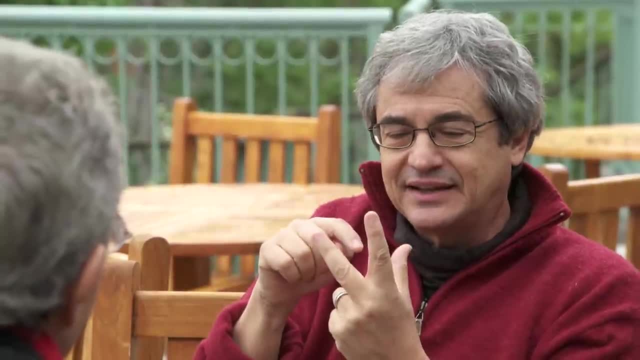 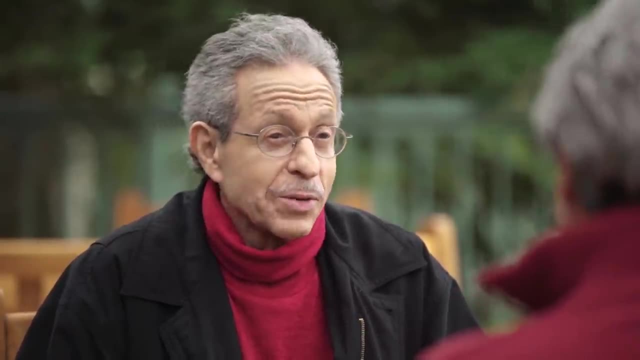 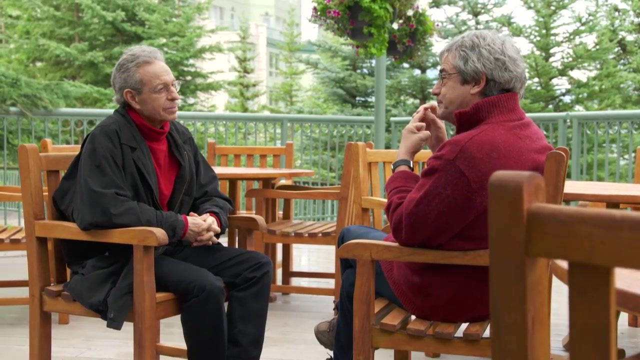 three has to be connected to the other, And none of this is very clear yet. What is the wave function of the universe Exactly? That sounds rather ambitious. The wave function of the universe is idea. that is in the third leg, So in the Can we do the quantum theory of everything. You see, my own take on that is that.